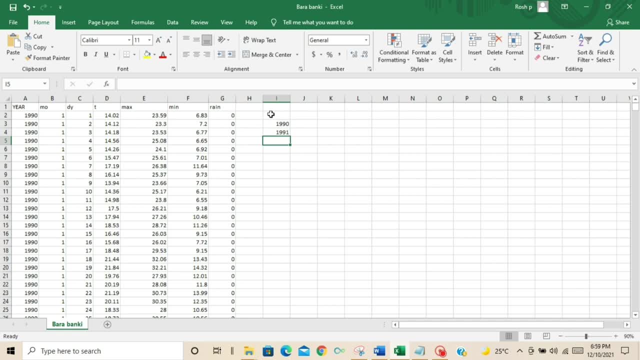 In this cell I am going to write the above value plus 1 so that I could get the preceding year. So I am just going to drag it So it will come till 21.. After this, once when the years have been sorted down, we are going to the column J on the formatting cell number 2.. 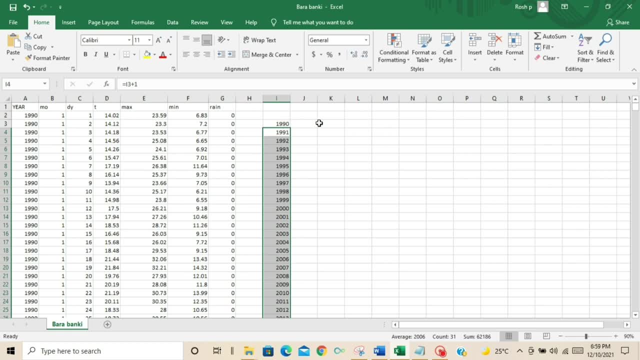 By this we are going to horizontally write the months, that is, January to December, in a numerical format to add it in our formula. So I am just going to use basic Excel functions, that is, 1 plus the prior cell value, to get the preceding values. 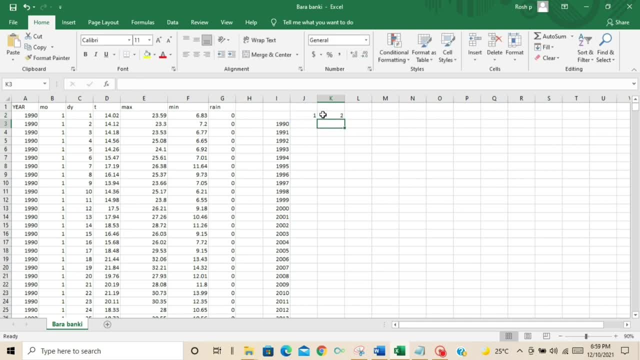 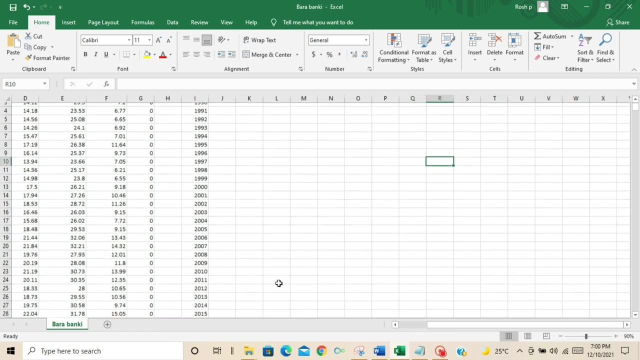 So it doesn't complicate the user's mindset also. So I am just going to drag it to U, alphabet U, so it gets 12.. So right now you just created a year and a column of year and a row of months. 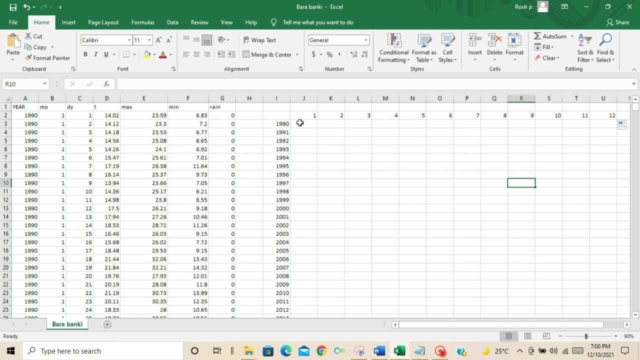 So now you have to use a formula Which will help you sort temperature values. So it is about average, if is, Just write, is equal to an average and on the last thing, you can find that average if is. So I am going to clearly explain you. what does this function do? 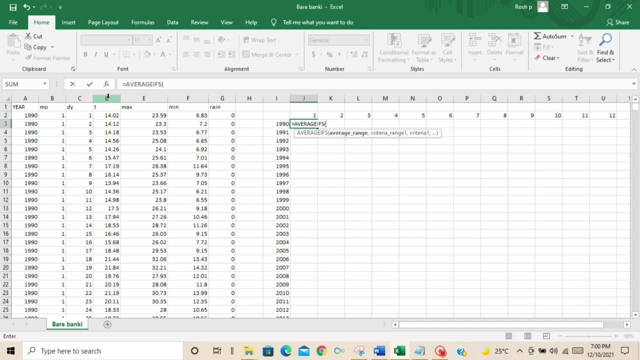 So I will just quickly just write it down. So I am interested in the column number E, So I will just write E is to E, So that I will also. I will also add dollar sign because I want the values of that column. 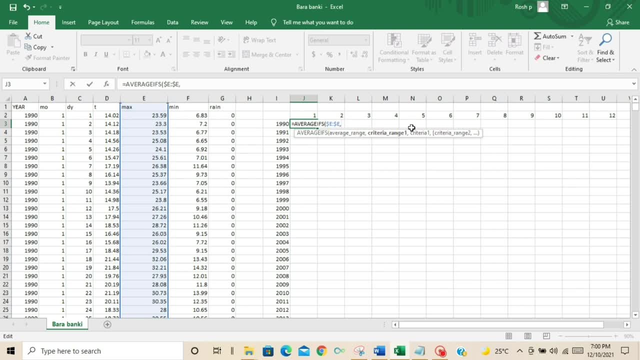 Then I am going to use comma. So maximum temperature. Next value I require is average year. That means the A column. Again, I am going to add dollar signs because I require the values in A column. Next is comma. After that I want to have that particular year. 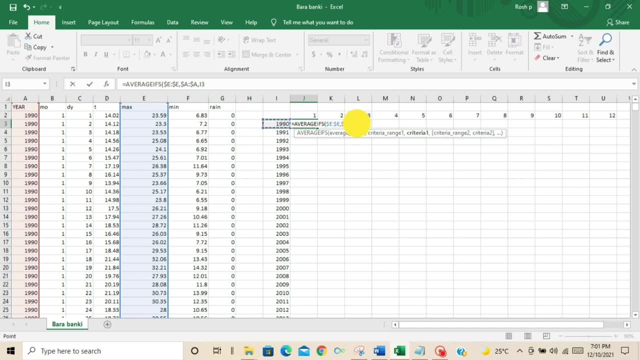 That is 1990, so that is I3. I will also add a dollar sign for this Comma. I want to also have the month. That is dollar sign B dollar sign. The column B value is required, So dollar sign is necessary. 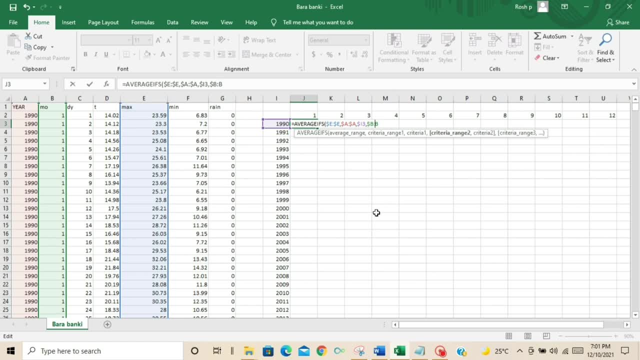 And then you have to use comma. Lastly, you require J2 value That is in the month. So I am going to use comma, And then you have to use comma. Lastly, you require J2 value That is in the month. 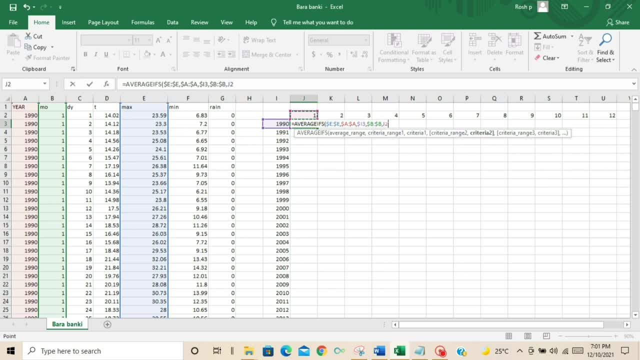 So that is in the month, So that is in the month, So that is in the month of January. That is why I am using J2.. So once you are done with this formula, you click enter And that is your maximum average value for temperature. 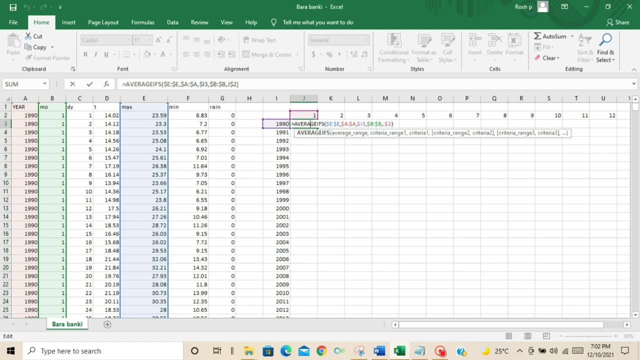 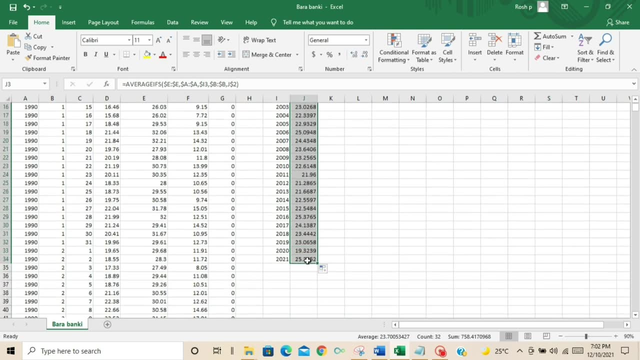 So we just do not need to do anything after this. We just have to drag down the values. And first I am going to drag down the values vertically. Just drag down the values vertically, so till 21 it will come. and then i'm going to horizontally drag it till you. that means till. 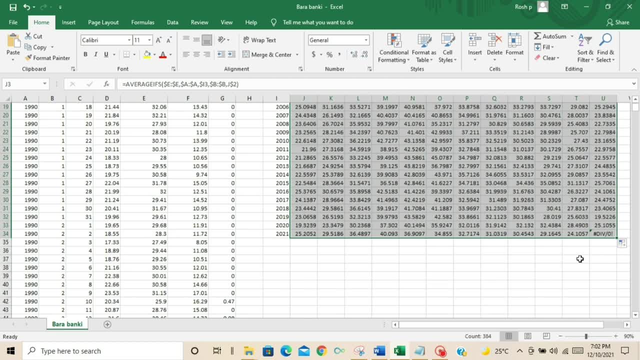 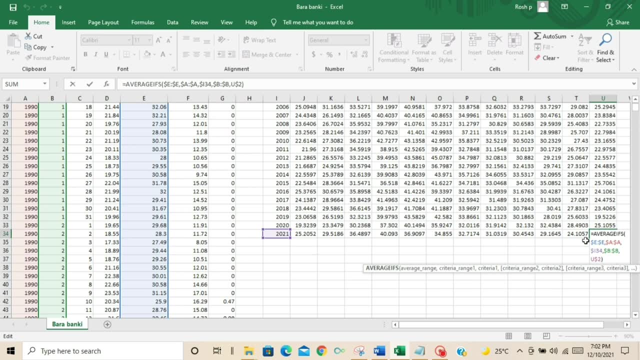 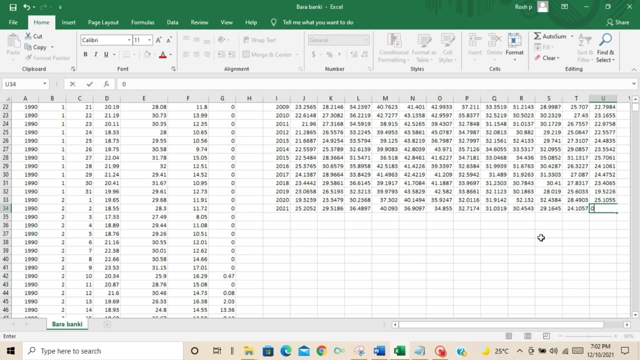 the 12th month, so this will give you a maximum temperature. now you can see there is a fault in that last column because that is 21 december. that value, 2021 december, and that value i have not written and i have not taken from the source as it was, as we are still in the month of november. so 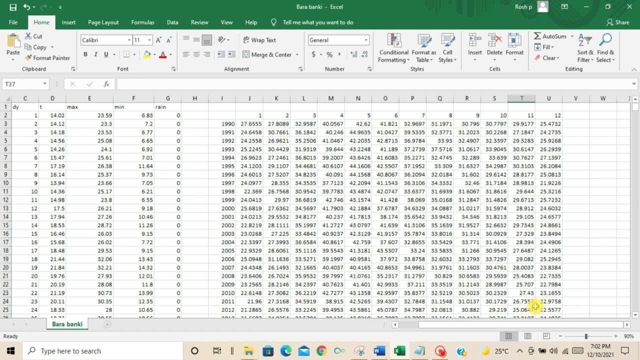 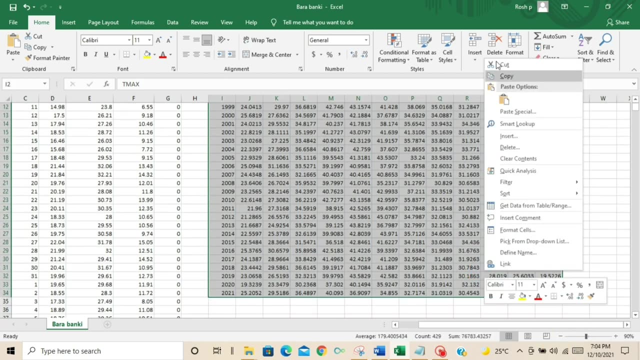 just, we just add zero. so that's all, guys. this is how your monthly mean maximum temperature is found. so i'm just going to write t max and i'm going to select the whole values to the next sheet so that i can use this current sheet for temperature minimum. so that's nothing, but i'm just going to. 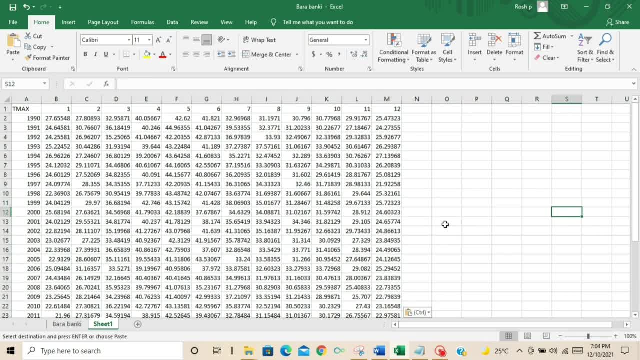 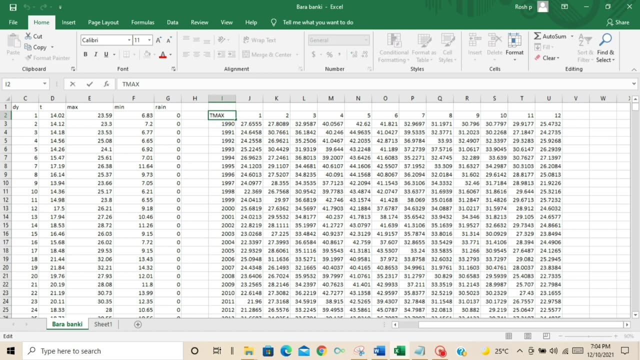 values, the second option. so that's it. you. it looks simple and clear. now for minimum temperature. we are just going to change few things, that's nothing. but we are going to just change our column. so where we had written e, we are going to write it as f, so f is in. 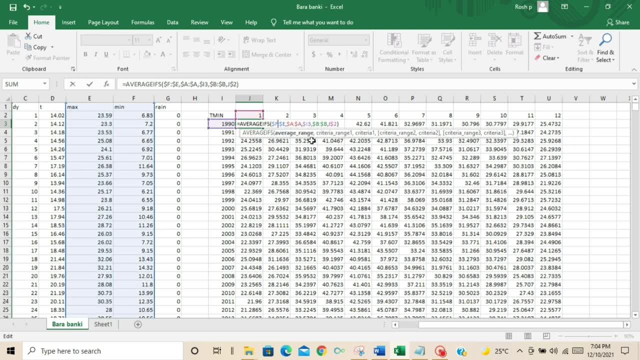 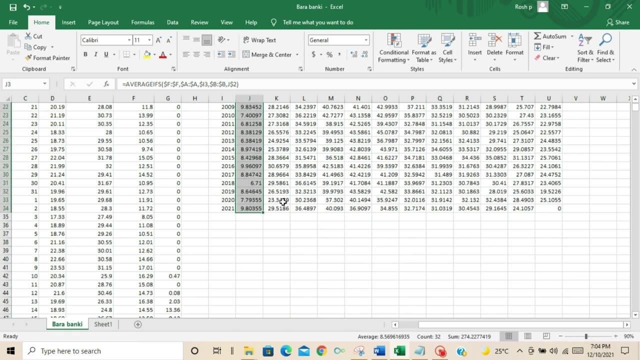 f column represents minimum temperature, because i have written it there. so, as you can see, when i'm showing u f' and i'm going to give it a max instead of tinha and the mtl and so on to found the t max variable here, so i'm going to keep it max so we get a maximum temperature of 38 celsius, so that 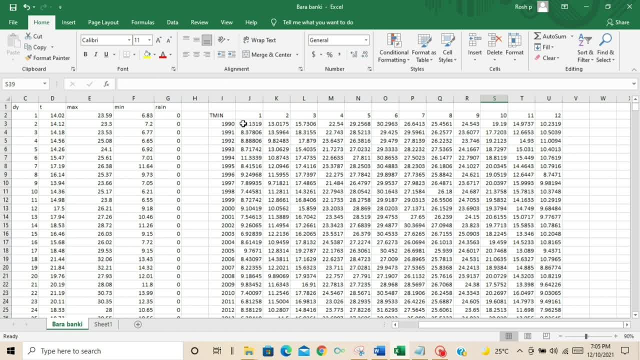 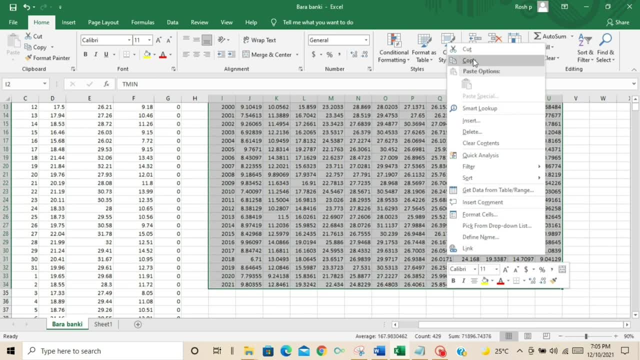 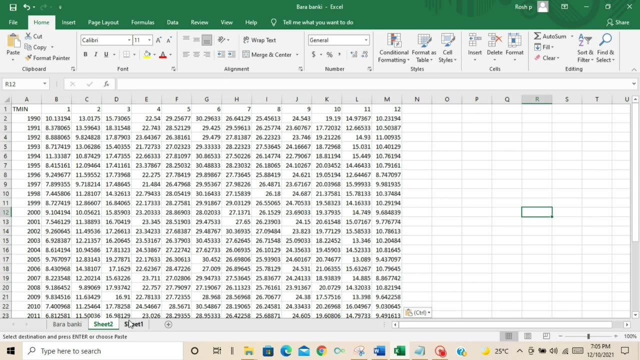 the sol in the unit 17 is equal to t k. you can double check roughly the content model on it. so, which is also important as well, and again, you can also provide status there too, just primarily for προ. so i'm just copying it, adding a new sheet, and i'm going to paste it by values. now i'm going to 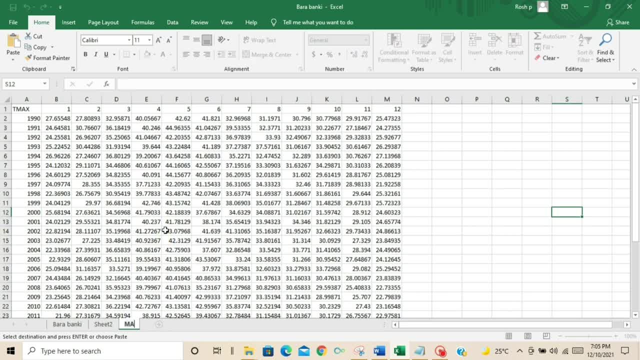 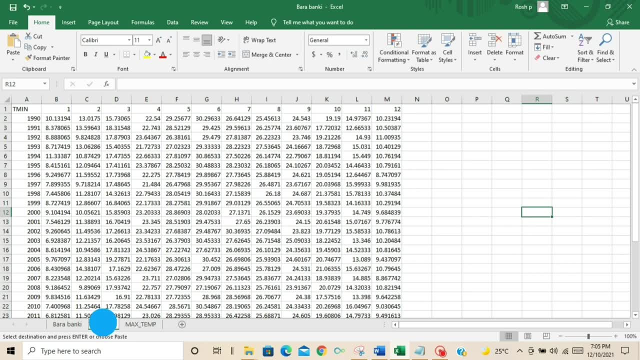 rename my sheets so that i don't get confused. but it's logically having sense that whatever higher values are maximum temperature and whatever minimum values are minimum temperature. so so that's all for this video, and rainfall data sorting will be done in the next video. thank you.